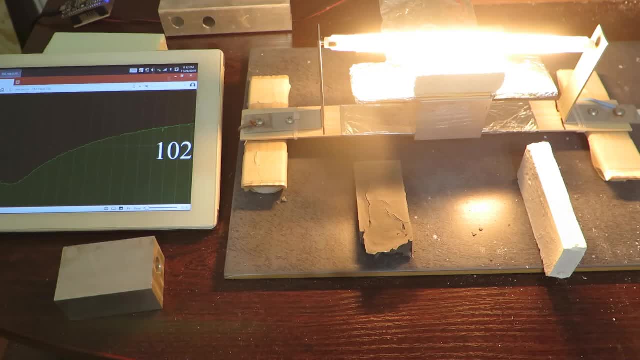 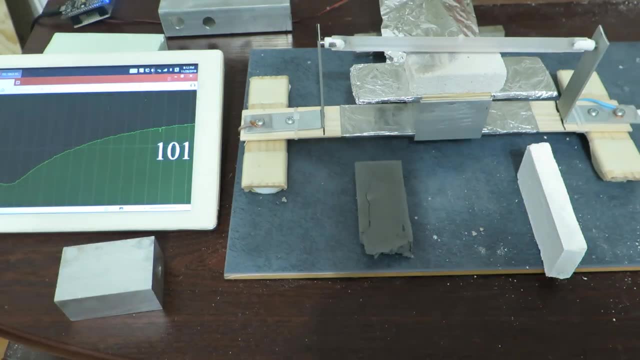 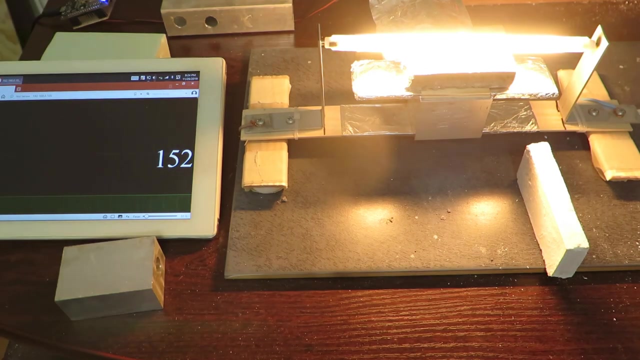 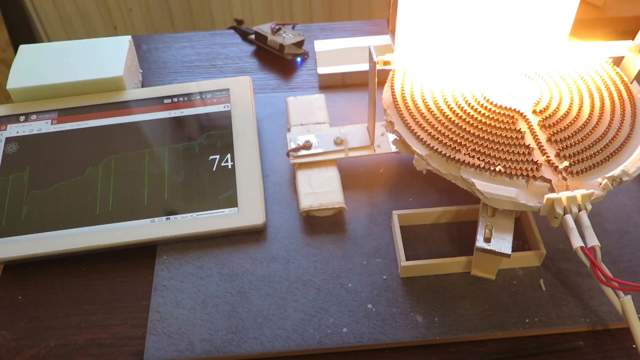 This sample is commercially available. pumice Also not quite suitable for high temperatures, but it has definitely some interesting properties. Now, high temperature sealant clay with calcium silicate- Very poor performance and very poor quality mixture. Finally, we measure our target temperature and 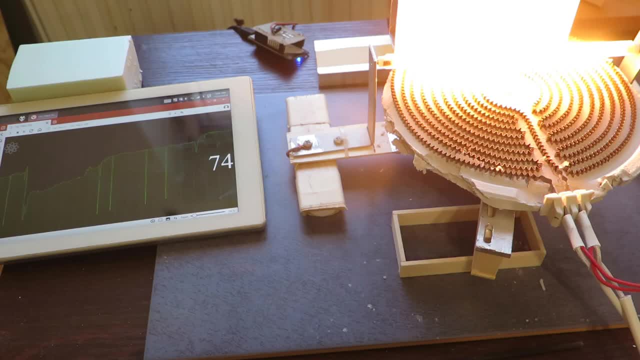 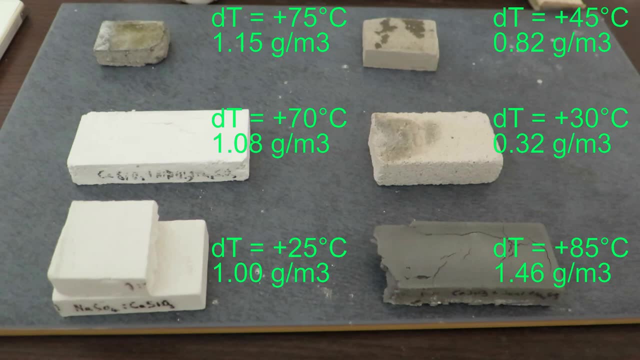 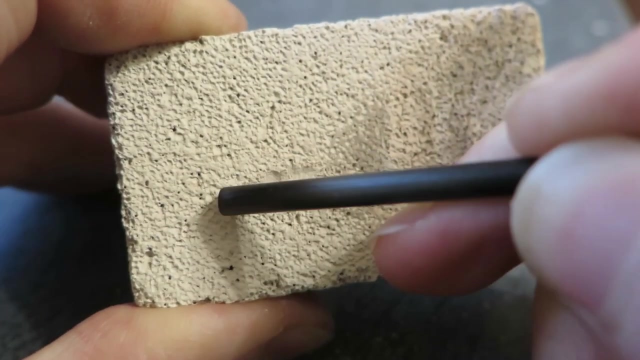 wow, I am impressed. Okay, so we are nowhere near Okay. so here are the bricks and approximate delta T from our target, along with block density. Now I don't know about you, but I really cannot see any trend so far. I guess let's move on to inspect some mechanical properties. 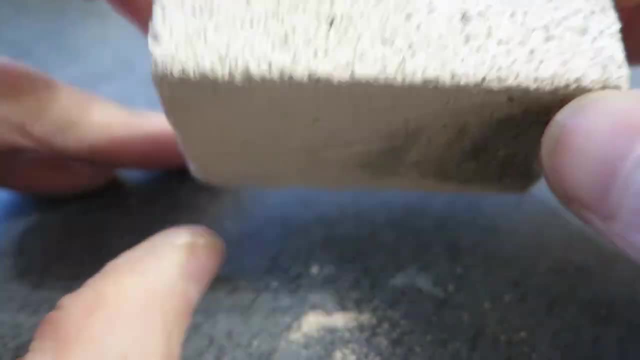 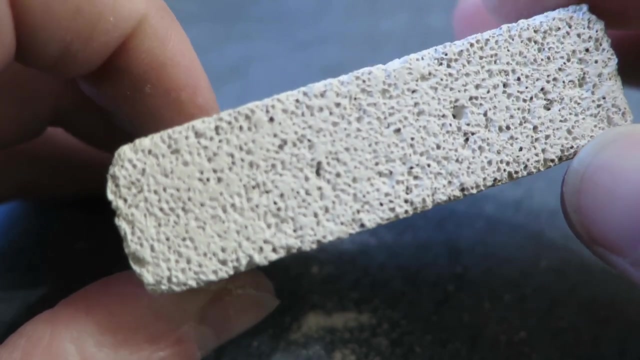 Famies, you probably know this material well. at least you can buy it in any supermarket. It's porous, quite soft and likely made of gypsum synthetically instead of volcanic rock. It has some strength, but it will likely disintegrate over time. 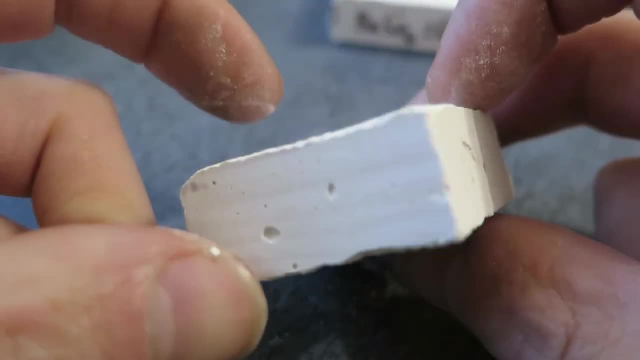 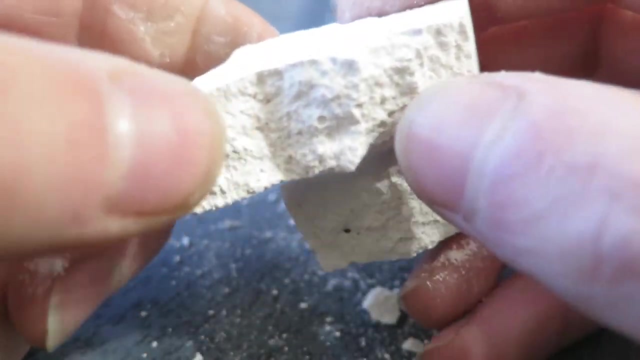 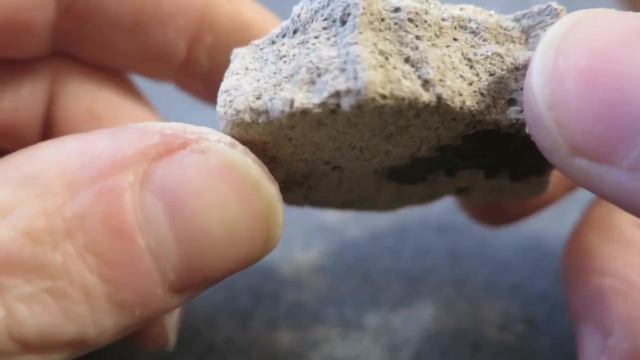 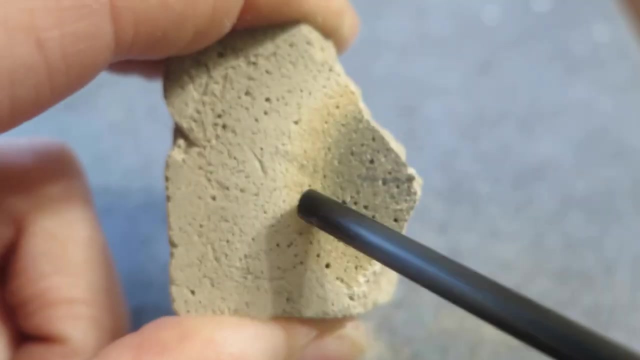 This is gypsum and calcium silicate mix. Similar softness and toughness, similar properties overall. In this block you can see the crust which has formed during curing. You can say that mixture was probably too wet. Inside is quite porous. that may helped thermal properties a lot. 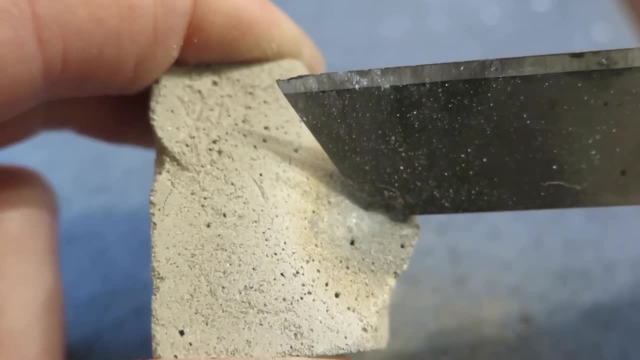 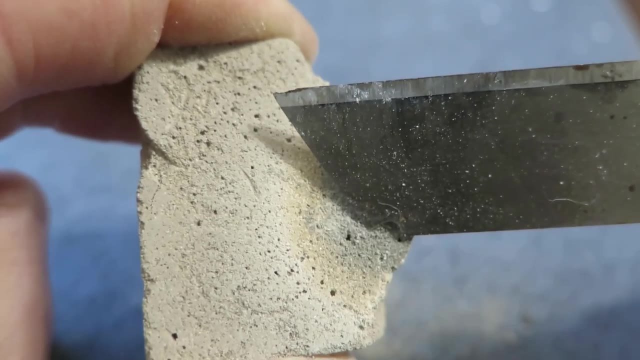 And here you can see the bottom part with the spot that has been fired with torch. It's interesting to see how soft this material is Now. as I said earlier, this is the same material as previous block, but fused with a bit more sodium silicate. 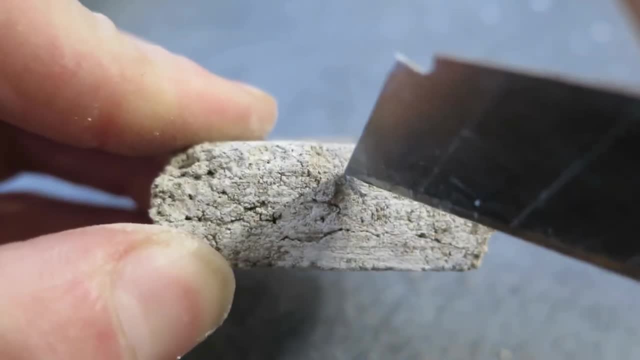 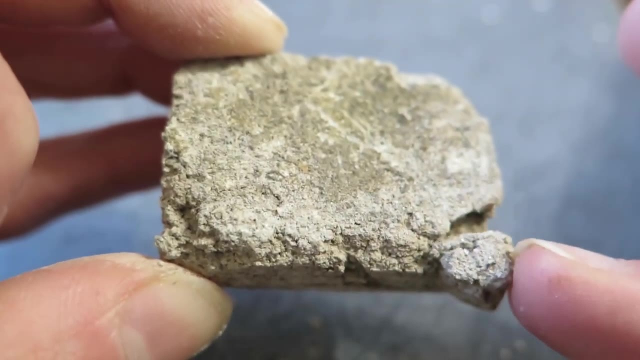 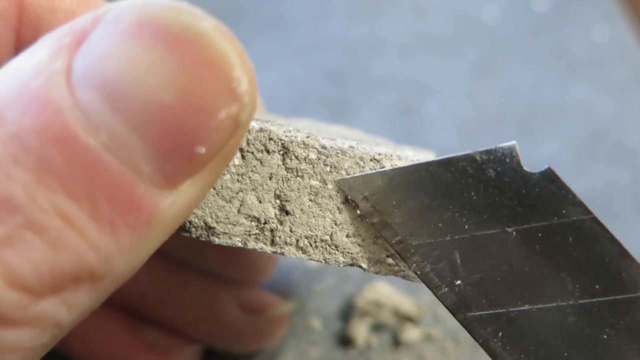 It has been fired from outside but with a small torch, so it's quite hard to harden this thick piece through. Considering how badly this thing holds together, it's quite difficult to work with overall. These white specks you see here are calcium silicate particles. 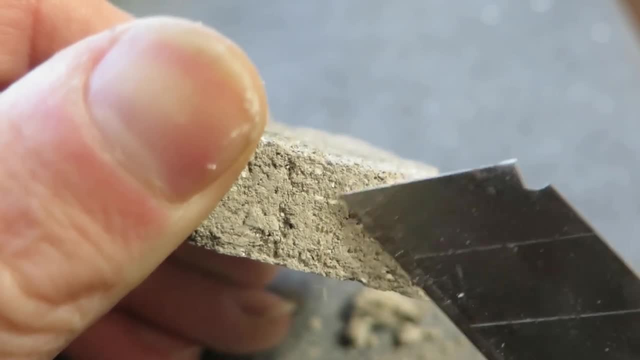 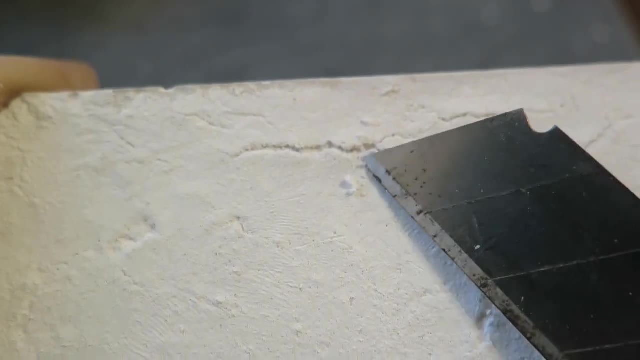 All bricks here are 50% calcium silicate. You can see that it's quite hard to work with. It's quite difficult to work with overall. This brick is alumina and calcium silicate. The crack you see here has been formed before curing by accident, so overall it has very 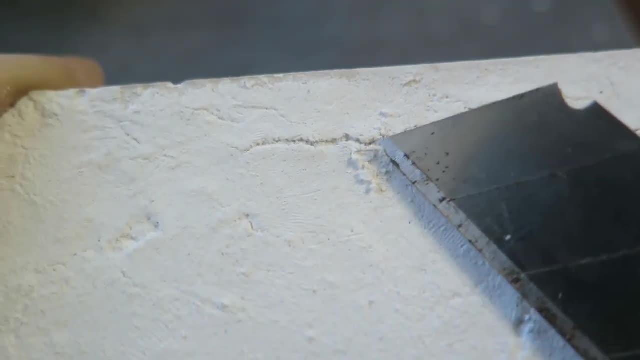 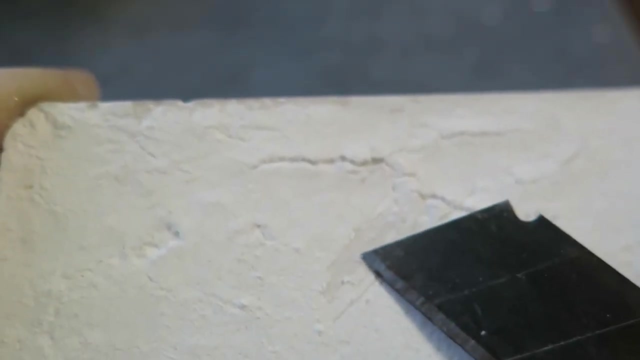 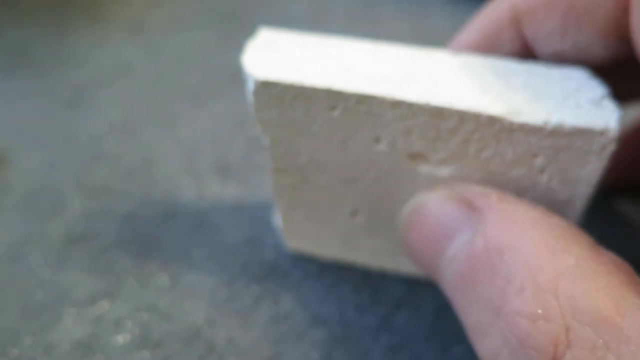 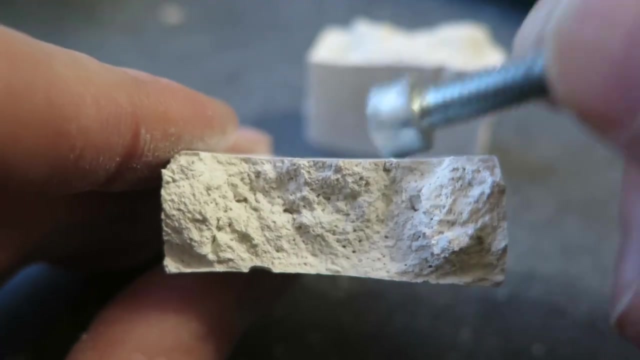 nice surface. However, this dust-like powder is most likely sodium carbonate that has crystallized. Nonetheless, underneath this powder is glass-like hard surface. This block broke easily, probably due to some crack. In the next attempt, much more effort was required. The inside is probably much softer and crumblier due to hydroxide preventing silicate to cure. 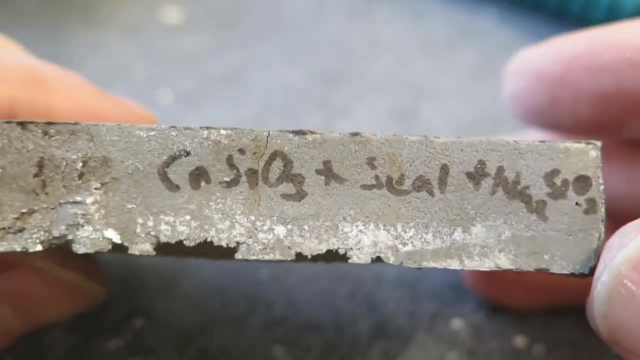 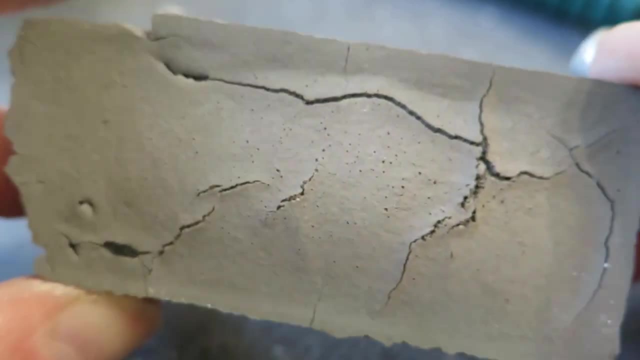 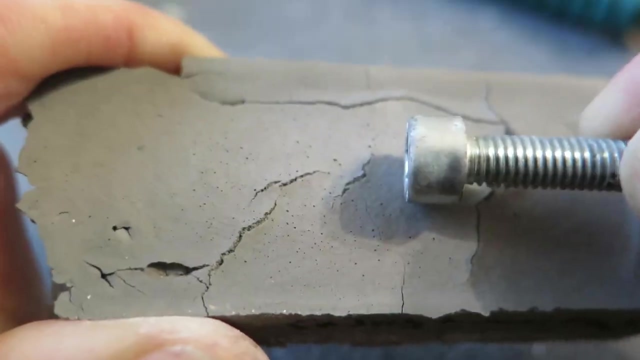 but it's still pretty hard. as you can hear, This block is made of super fine clay and calcium silicate. When surface of this clay hardens, it greatly inhibits further curing, so it's not too usable material overall, But it is super hard and abrasion resistant. 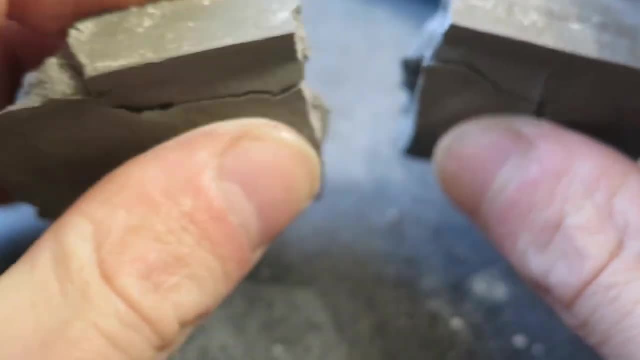 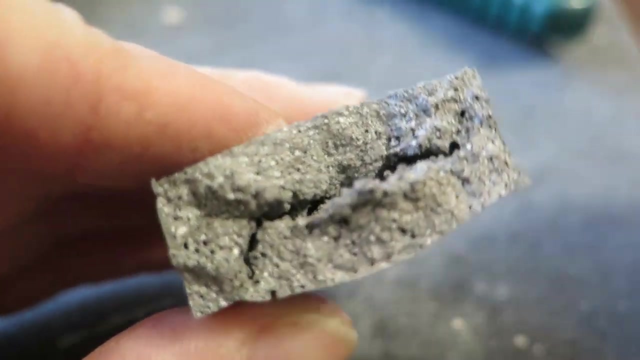 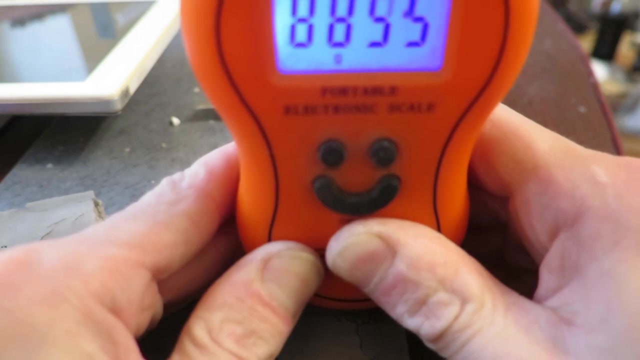 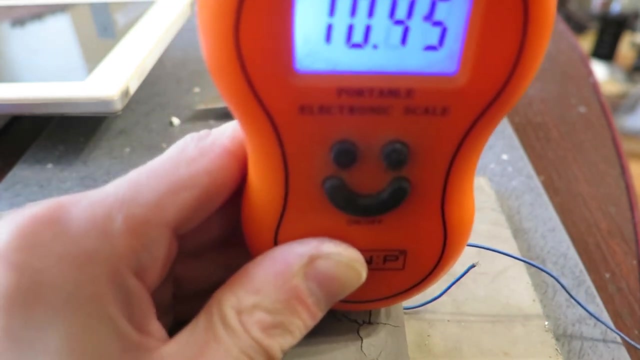 This cavity inside is caused by steam pushing on already hardened crust and it is pretty much unavoidable. In this last segment, I will measure how hard you can press on these blocks with portable electronic scale before they shatter. So this sealant clay block can take 15 kilograms. 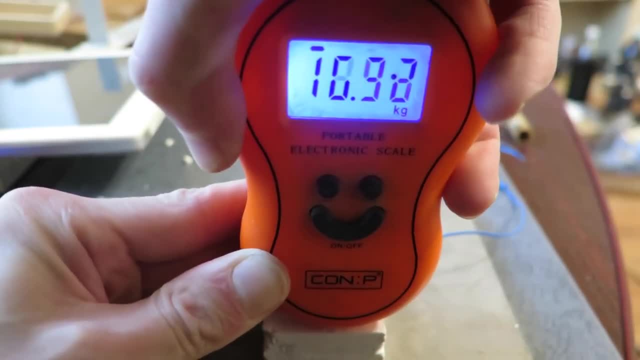 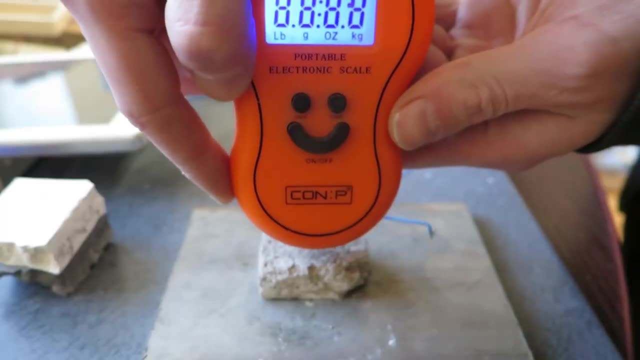 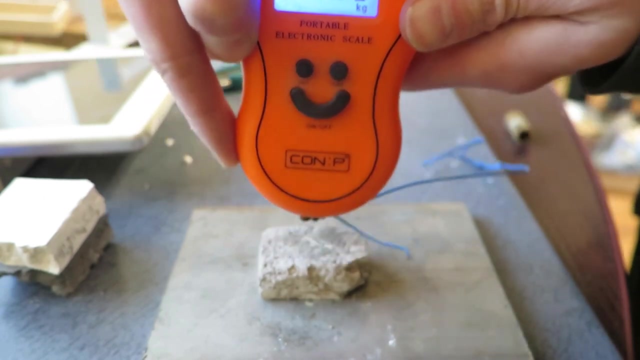 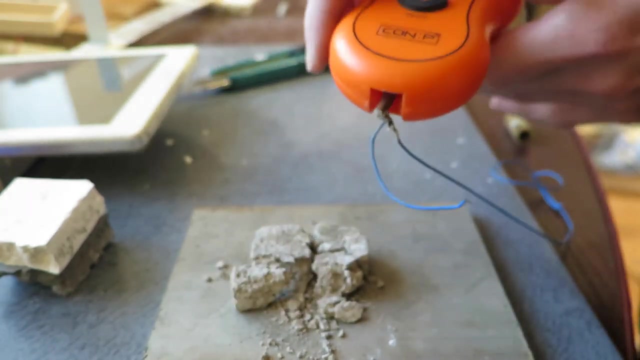 Very tough material: Aluminum block, 15 kilograms. no impression: Good stuff overall. This is mortar Getting quite inconsistent readings, probably due to varying hardness of the surface. And again mortar About 1 kilogram of force to break this. 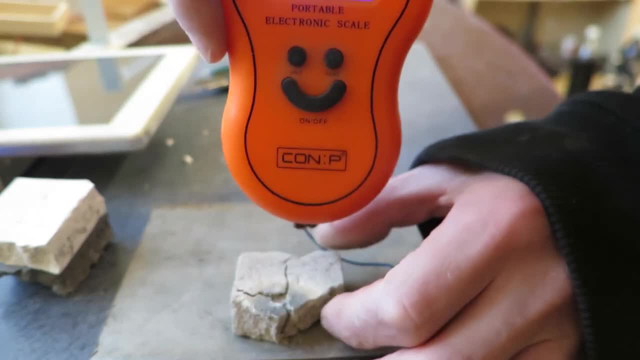 And again mortar About 1 kilogram of force to break this. And again mortar About 1 kilogram of force to break this ata block. It takes abour 15 kilograms to shatter. First. I will put these blocks here. 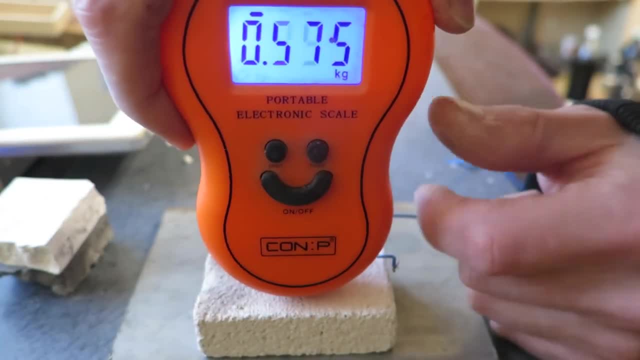 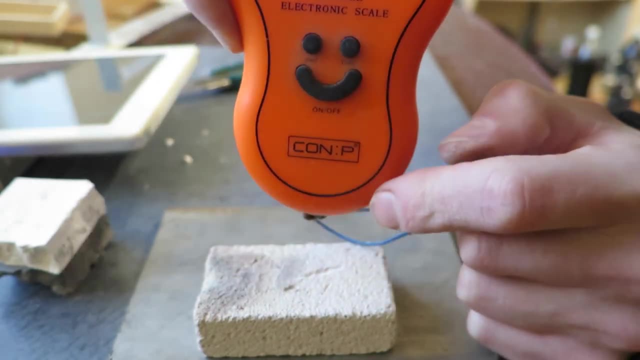 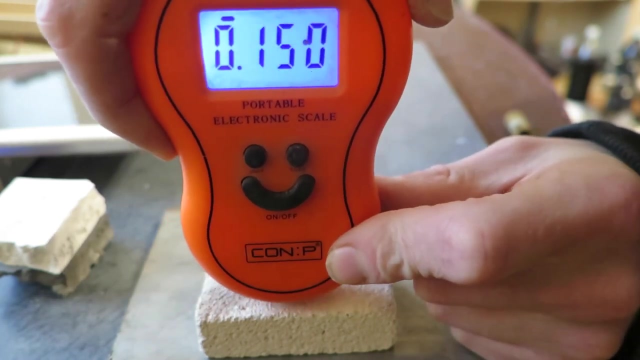 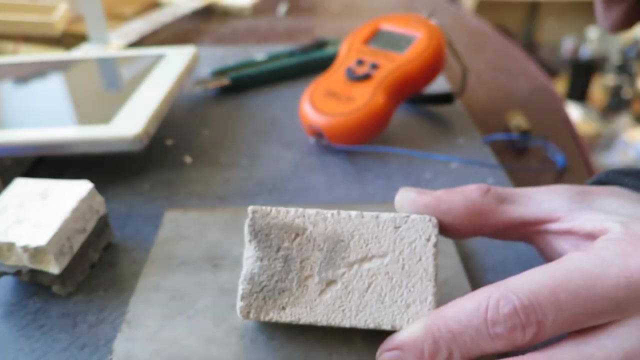 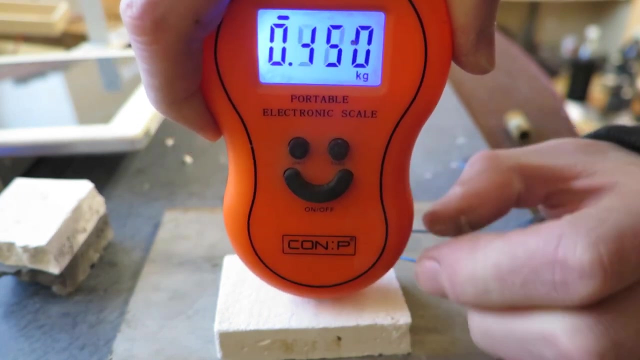 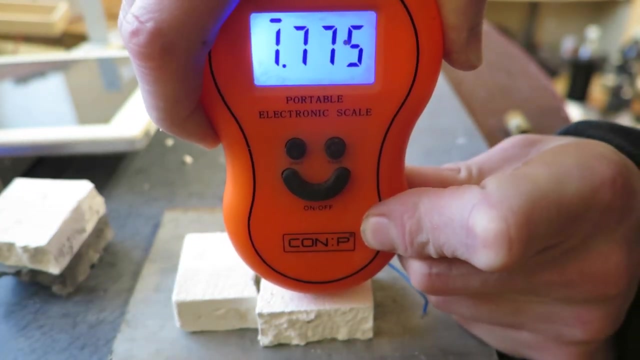 There is impression, so the integrity can be improved with some reinforcement or maybe hardening of the inside. Now this is impressive, how such brittle material can withstand so much pressure and basically, at one point Very good. And gypsum Not good, Better. 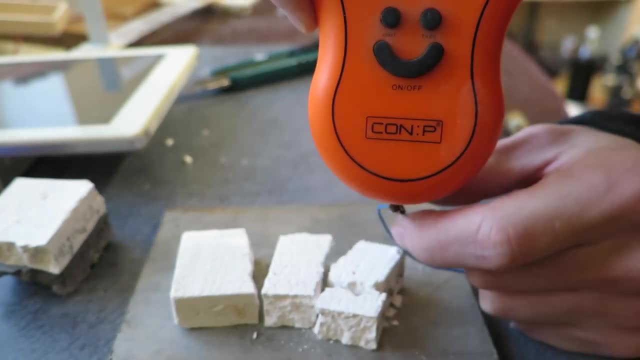 And impressive. So conclusion: Yes.